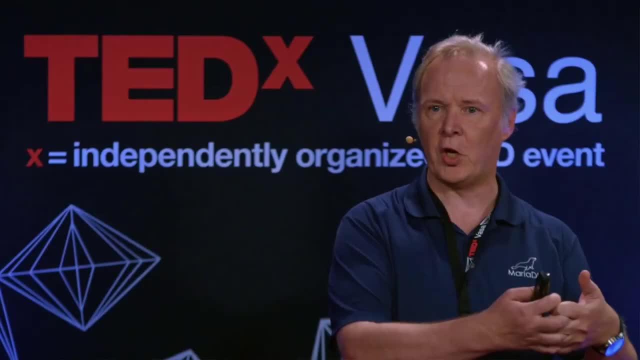 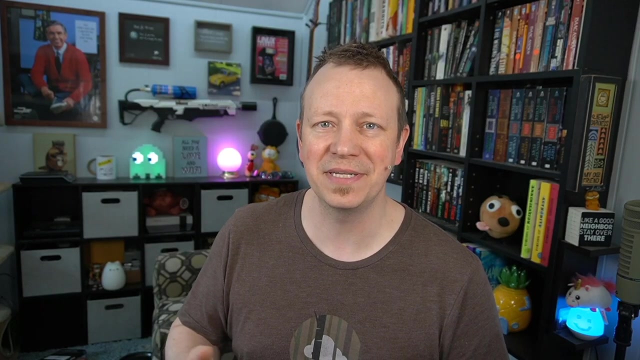 they were both created by the same person, Michael Widenius, and I probably pronounced his name wrong, but he has two daughters. He has Mai and Maria, And so the databases are literally named after his daughters, which I just thought was cool. I assumed Maria was named after somebody. 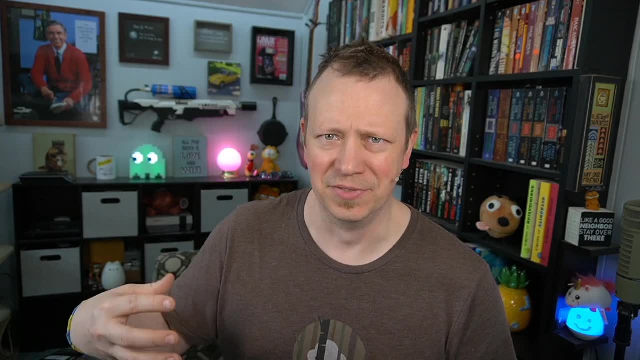 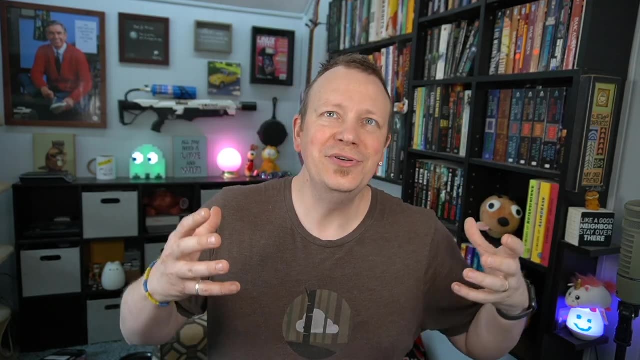 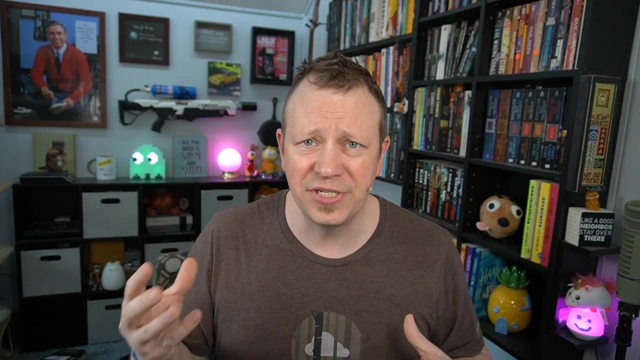 but I thought the Mai in MySQL was like you know, like this is my database open source- blah blah blah. Nope, It's after his daughter named Mai. Anyway, there are two basic ways to back up databases, and this is something you should do regularly. I want to show you both ways and how to restore. 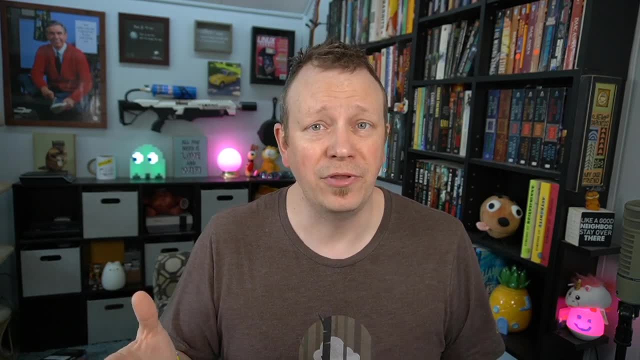 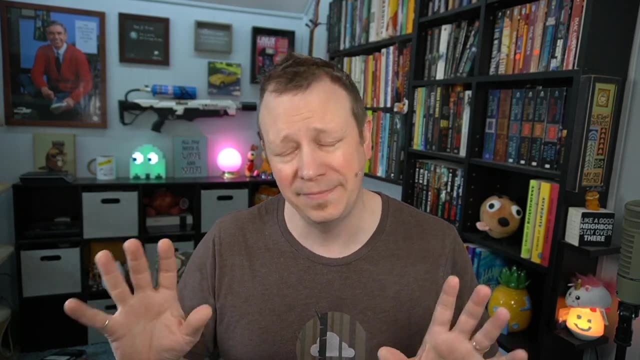 and that sort of thing. but your situation, you may want to do both, You may want to do both types of backups, You may only want to do one, You may want to mix it up and do like one regularly and one occasionally. however you go about doing it, It's important that at the end of 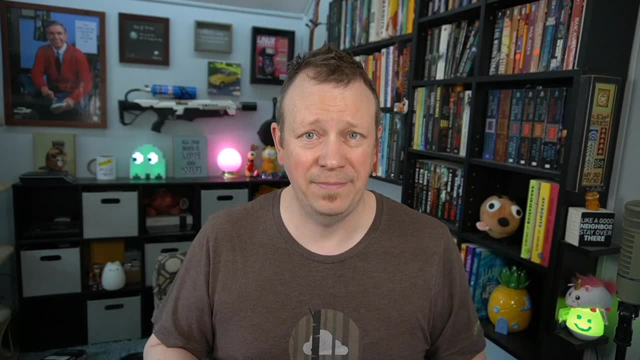 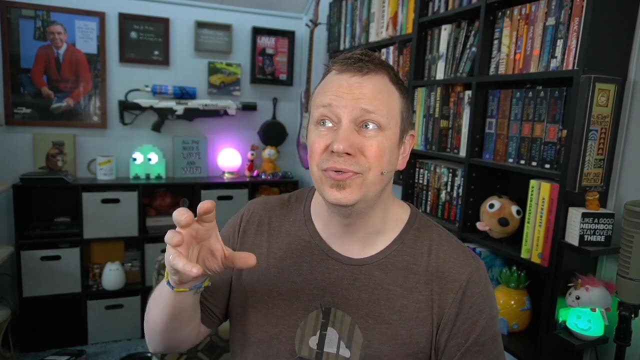 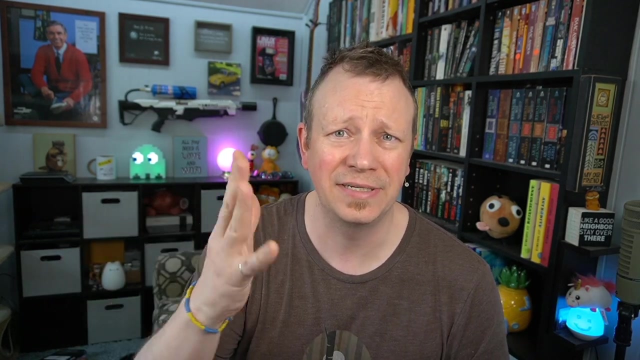 this video. you feel comfortable backing up databases. And now I should confess I have a dirty little secret and I know that I have showed you how to have Docker share, uh, Docker instances that are serving out databases using the Docker network- stuff in real life I actually don't like. 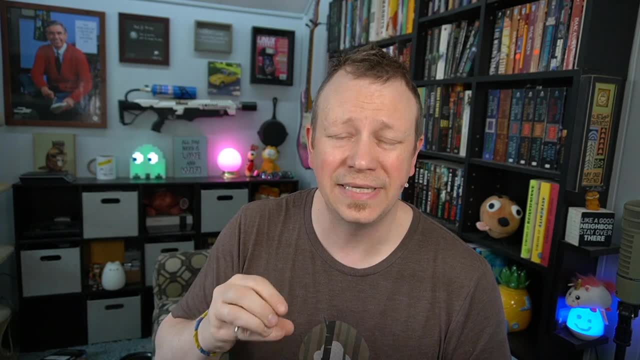 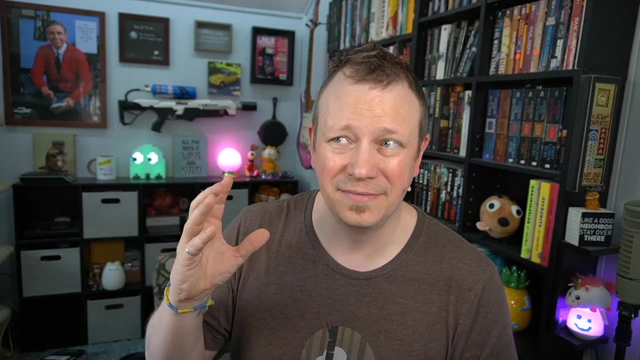 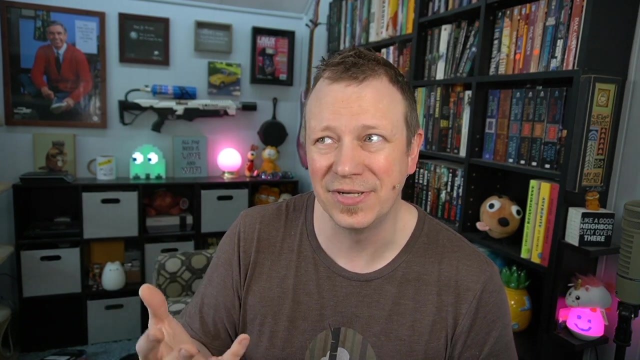 to uh host my MySQL or MariaDB uh stuff in a Docker container. I like to have one central server, a full-blown uh machine, that I can log into and run backup scripts on and stuff like that And then point all of my instances to that. So I'm sorry if I misled you, but it's you know. 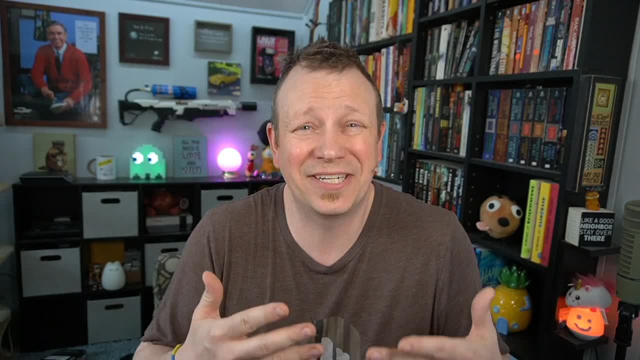 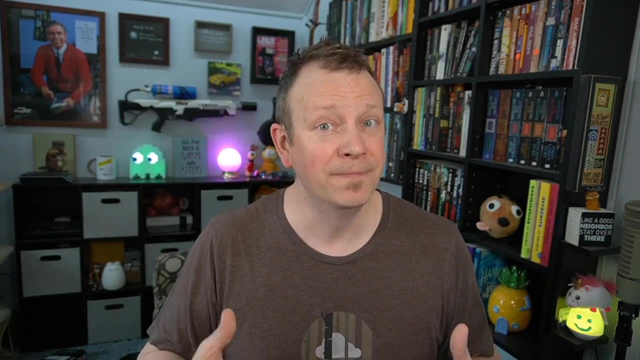 a lot of people really want to share MySQL databases inside Docker, So that's why I've talked about that before. but I like to have, uh, MySQL and specifically MariaDB server that all of my containers and other stuff point to anyway. So we're going to be looking at a machine that is 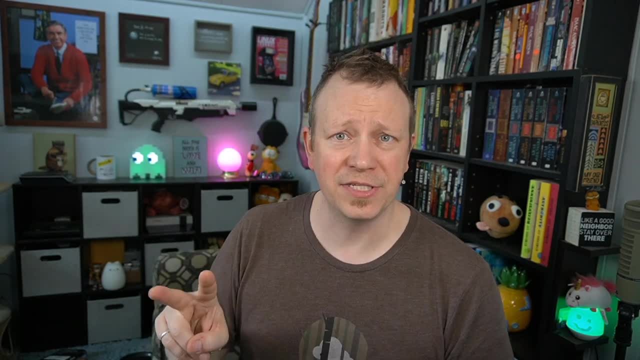 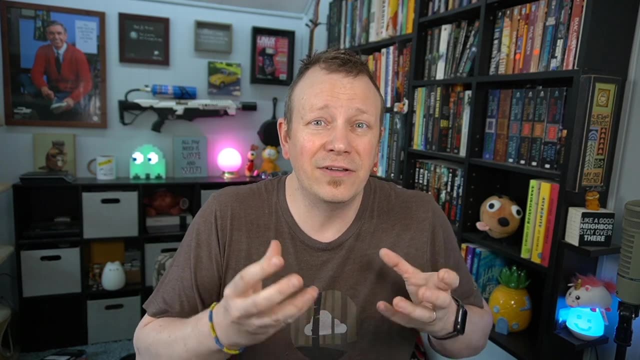 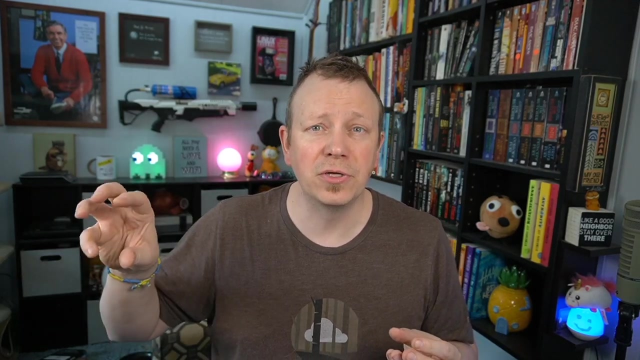 literally running MariaDB. Now the two backup methods are a physical backup, and this is where you literally take a copy of the files in the var lib MySQL folder- all of those files- and create a snapshot copy of them. So if something goes wrong, you can restore those files. Now it's possible to restore like one. 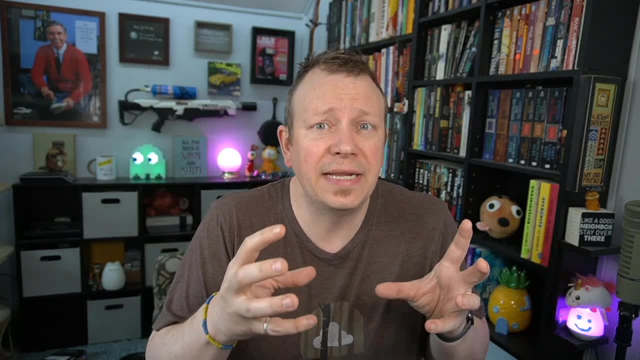 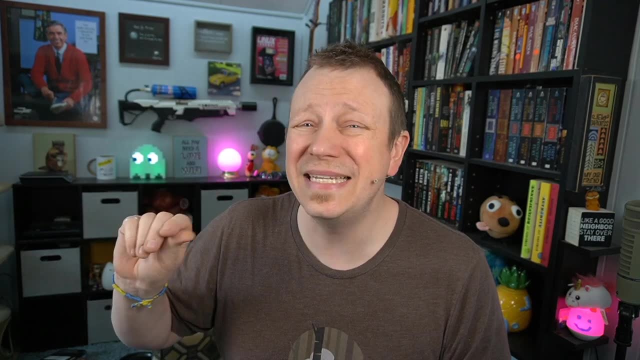 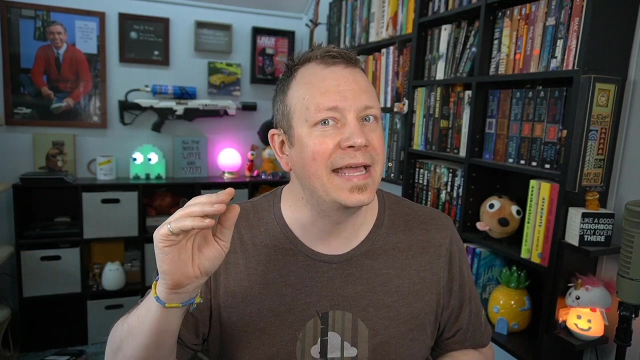 folder which is one database, but you're basically taking the entire database, with all of its users and all of its stuff, and making a complete snapshot of that folder. Now, the reason that is easy as using traditional file backup software is that it's a live database and those are. 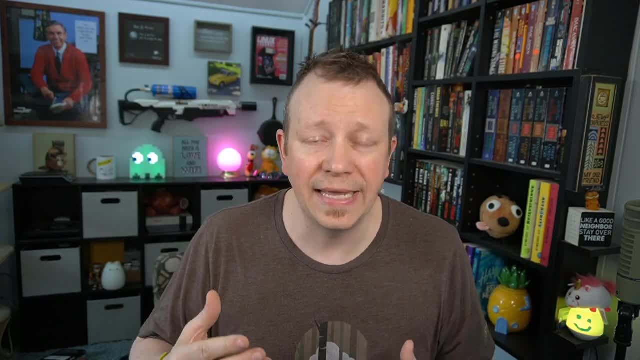 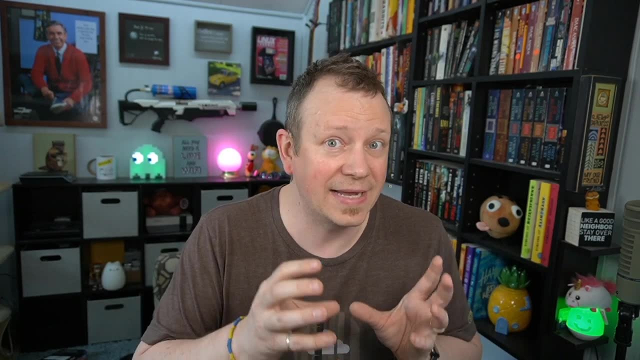 constantly being written to. So there is, thankfully, a tool we're going to look at that will uh, kind of I don't know, I don't know what it does, It does some magic stuff in with SQL so that you can make a copy of the file. They're not worried that like it wasn't written to or it was open or 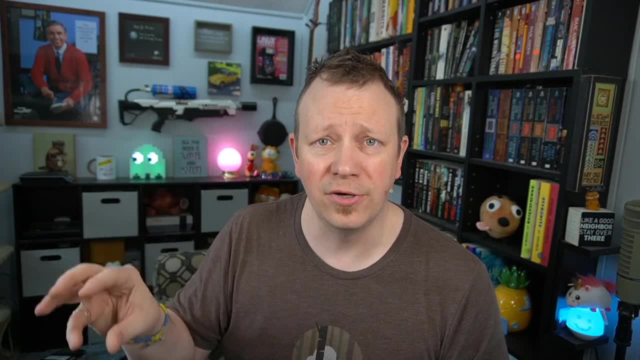 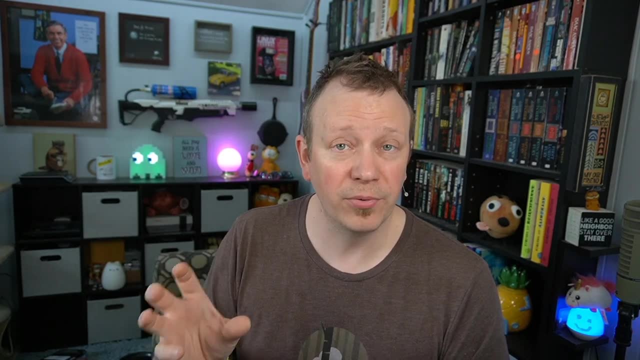 you know it gets corrupted or anything like that. So we're basically going to make those uh physical copies using uh, that physical uh backup method. Now there are some pros and cons to this. The one of the pros is it's. 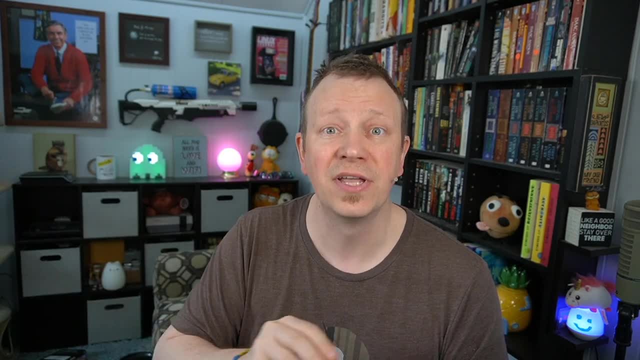 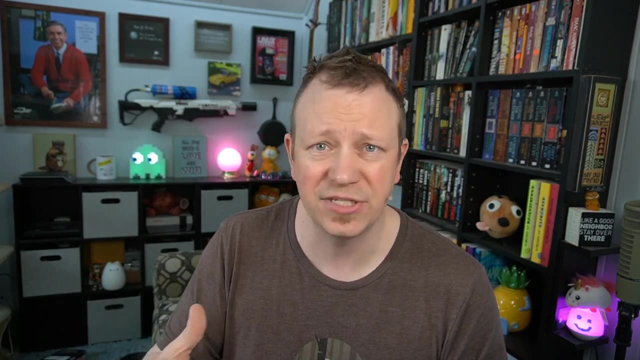 extremely fast because we're just copying the actual files off of the server. We're not using SQL to like pull data back and forth. We're not making a lot of database calls or anything. We're not making any database calls- Well, maybe it does- to pause the data so you can copy. 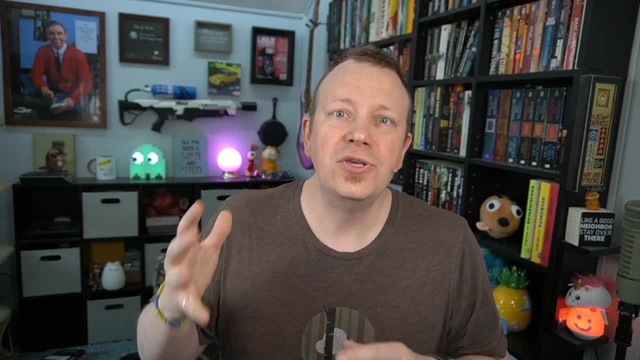 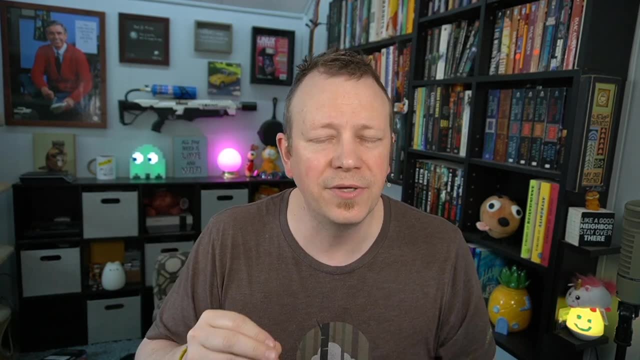 It's very fast, Okay, So it's really really quick. Um, you can, in addition to the snapshot you have, if you have digital logs enabled on your Maria DB or my SQL server, you can actually go and get all of the transactions since you backed up to right. 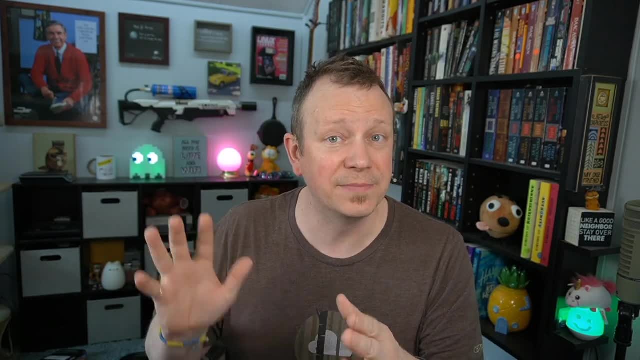 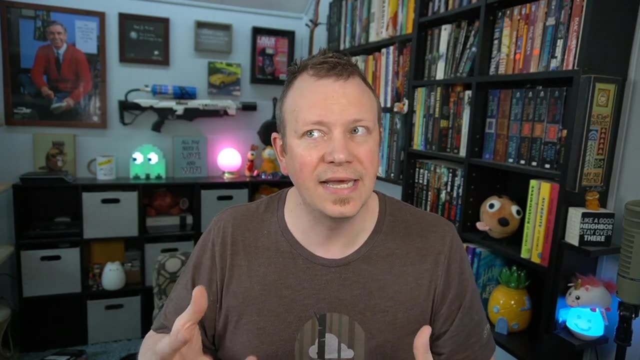 before it crashed. That's beyond the scope of this video, but it's possible to actually restore, up to the minute before it crashed, all of the stuff into your database. So it's a really it's nice to be able to do that, Um, but there are some cons. one: it uses more space. You're literally taking a full 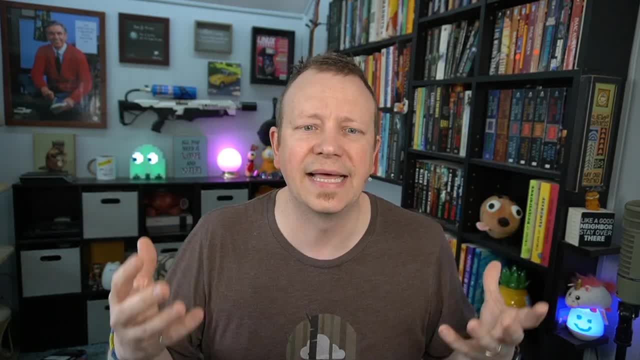 copy of everything there, So you it. it takes a lot of space to do that, And one of the biggest cons, though, is that it's really really fast, So you can actually go and get all of the stuff, Um, 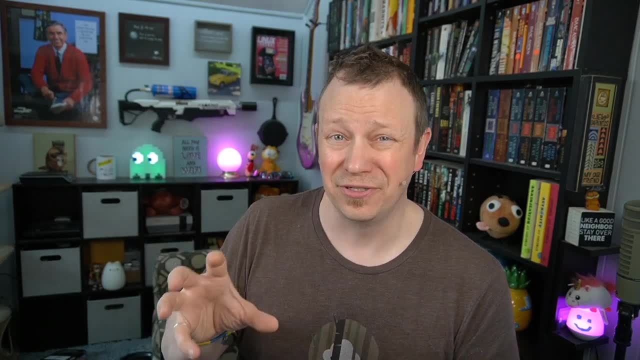 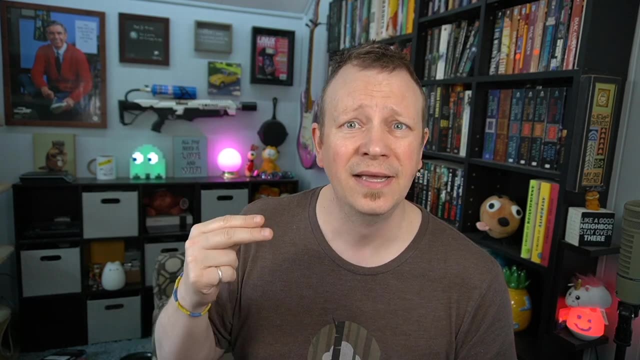 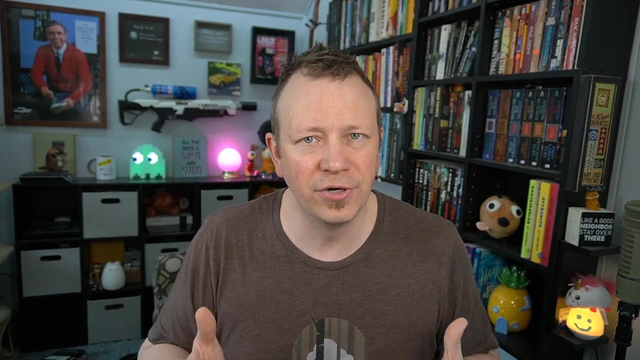 is that this is not a good way to migrate from one server to another. You're going to want to use the exact same server type, the same version. Uh, this is basically a disaster recovery type thing. This is not a data migration way, because something's changed between versions and you're 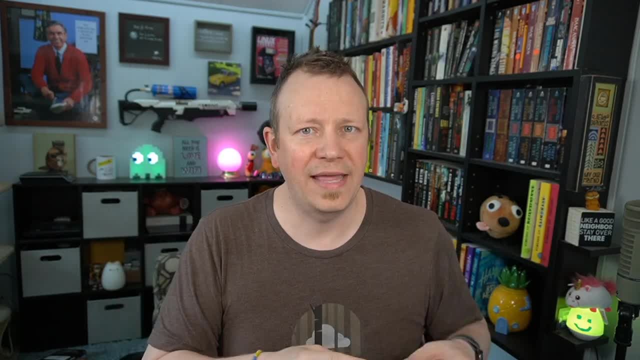 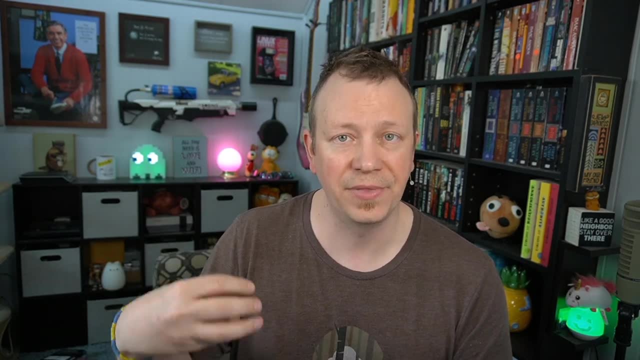 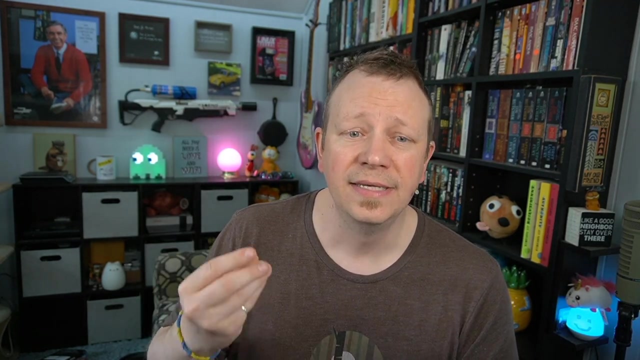 literally taking the files off the hard drive and that's what you're backing up. So that's. a con is that this is not a data migration from one to another. This is a way to restore if something goes horribly, horribly wrong. And now the other way that you can back up- uh, my SQL and Maria DB. 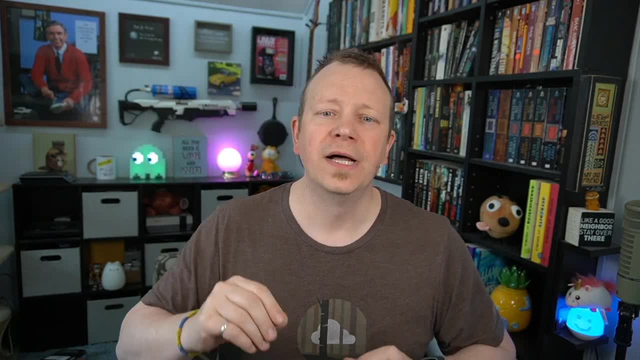 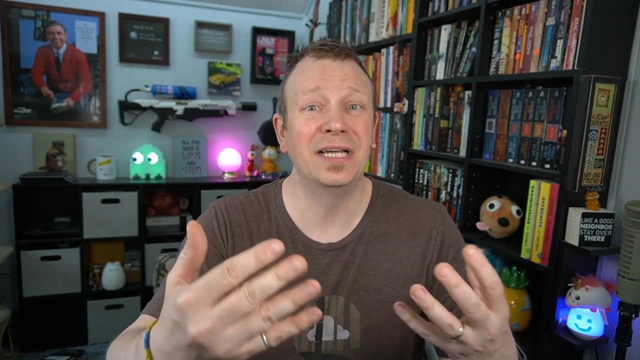 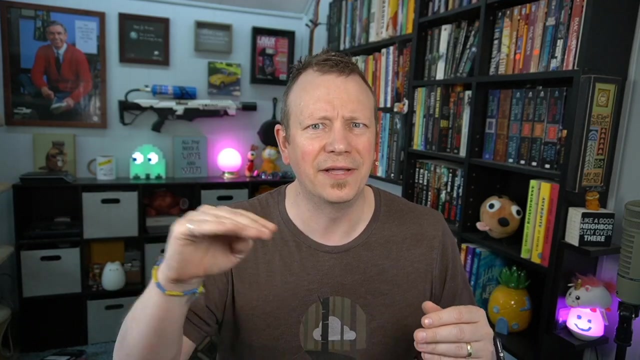 databases is to use a logical backup. Now, a logical backup just makes, uh, an SQL file a SQL file and it uses my SQL dump and it just dumps all of the information from the database into a list of: basically, it's a, it's like a list of commands to tell the database. 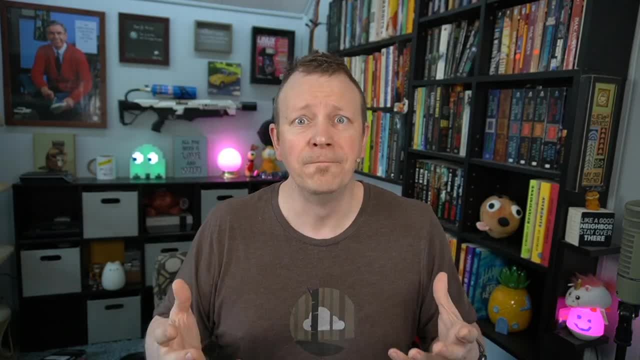 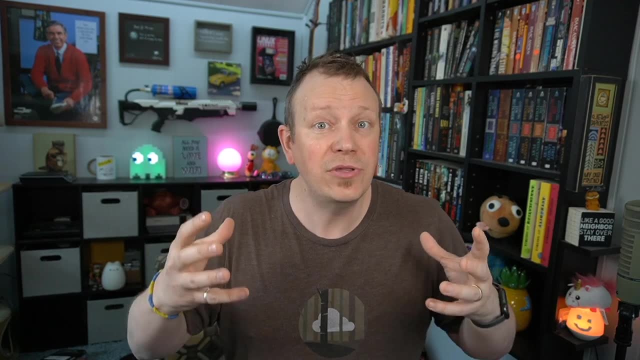 how to rebuild itself from scratch. It's really cool, Um, and it has some great advantages. Uh, one of the pros is it's very, very flexible, And this is how you would migrate from one database to another. You can usually even go like between versions, and you can. 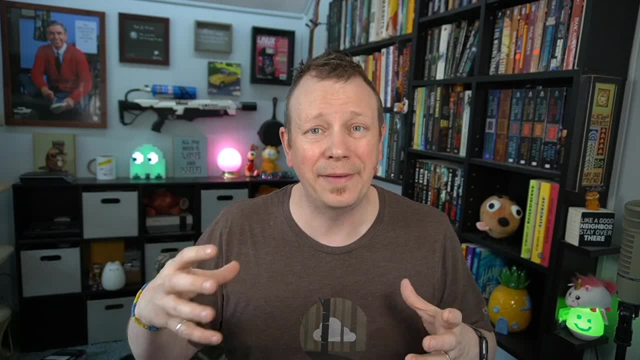 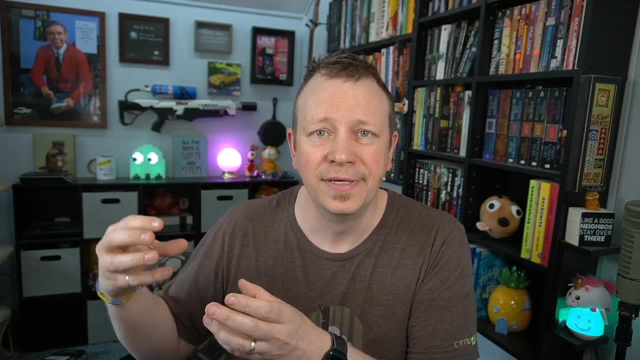 uh, maybe between my SQL and Maria DB. I mean again, these are just SQL commands, so you have the ability to take it to another whole server. import the SQL, the SQL statements, and it will create your database or databases. uh, just like that. 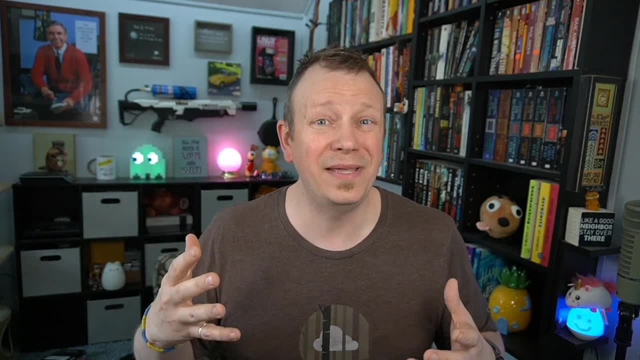 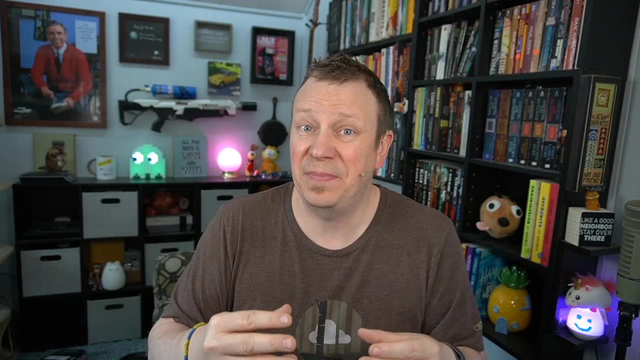 So that's a big pro. Um, another pro is that it can be compressed right. This is like a text file on how to create a database. You can, like G zip it on the fly to save space for your backups, which you should have. 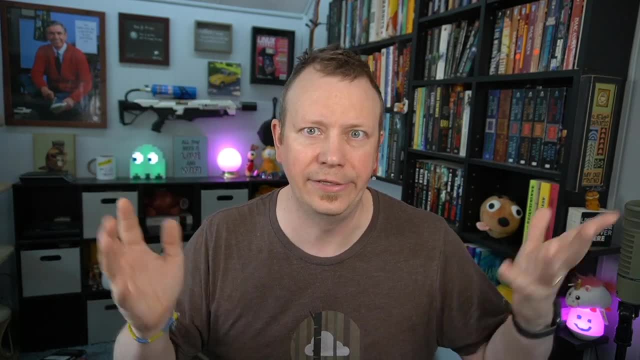 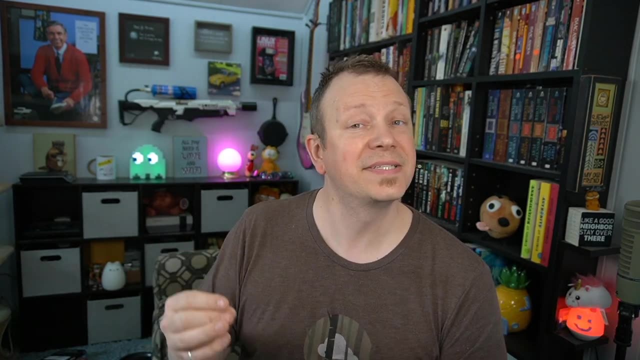 multiple backups, you know, going back however long your backup procedures tell you that you need to do. Uh, so that's really good. Um, there are some cons, though. It's very, very slow, and it's slow because you are literally doing SQL calls to the database for every single thing. 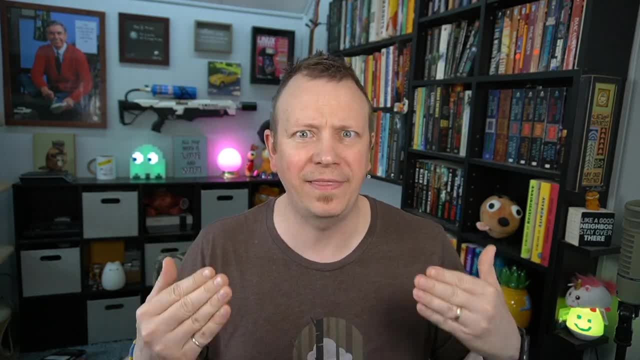 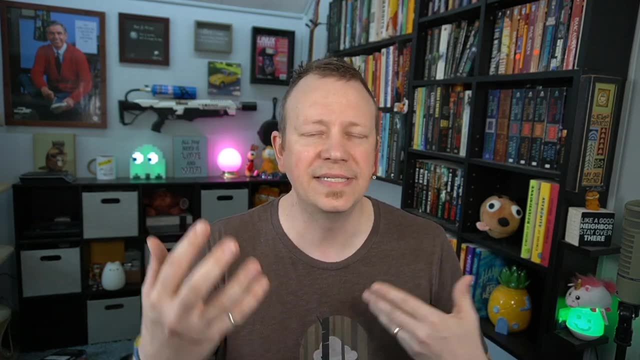 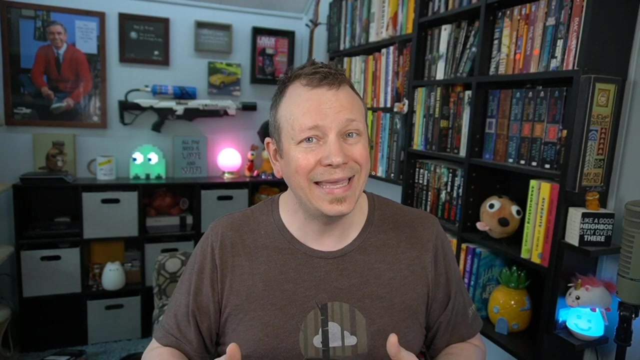 The database has. you're saying: okay, database, tell me everything, you know about everything, and I'm going to write it down. And so the database software, the server, crunches through its entire everything and then writes it to a SQL file for you. So it's not very fast, It's kind of slow, And that's the other con is 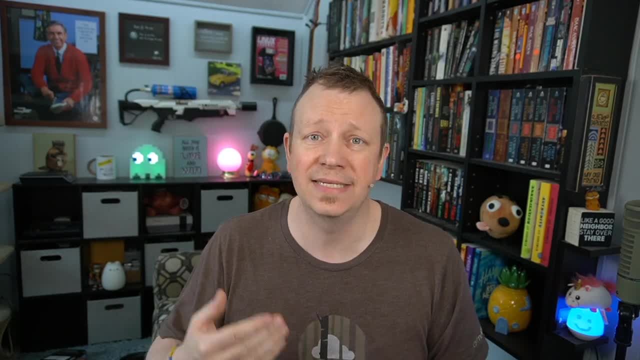 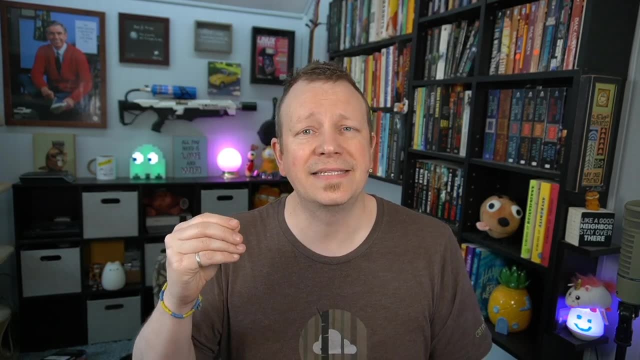 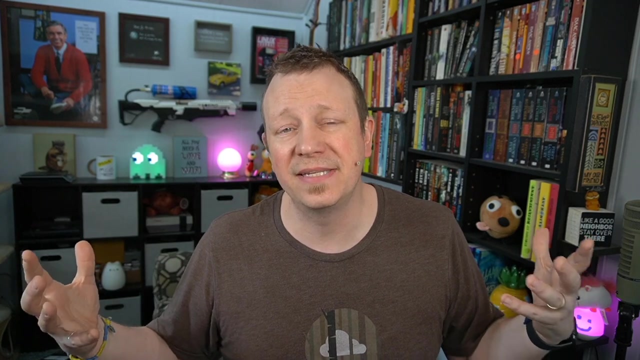 it taxes the server pretty heavily because you're making constant hammering calls to the SQL server And because of that it means that the final con is: it's not terribly scalable If you have a really, really big database or multiple fairly large databases. doing a MySQL dump or a logical backup is not a great idea, because the time it takes to create and or restore that backup are just going to be so long. Sometimes you won't be able to complete the backup before it's time to back up again. So there are pros and cons to both, and just 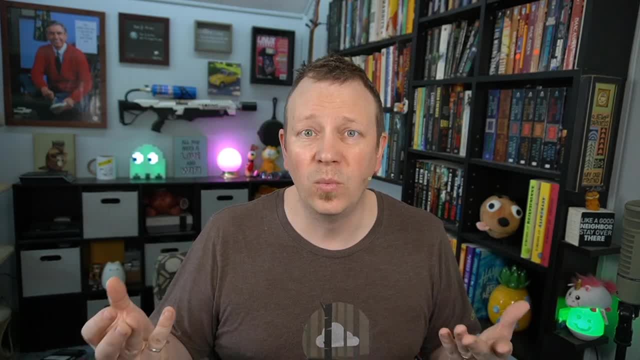 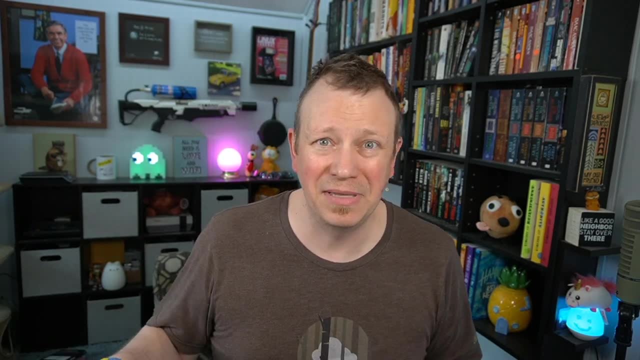 you know, weigh what your needs are and and that's how you decide what kind you want. or you know, maybe you want more than one kind and you want multiple copies. and you know, maybe a MySQL dump every so often, I don't know. whatever makes sense for you. 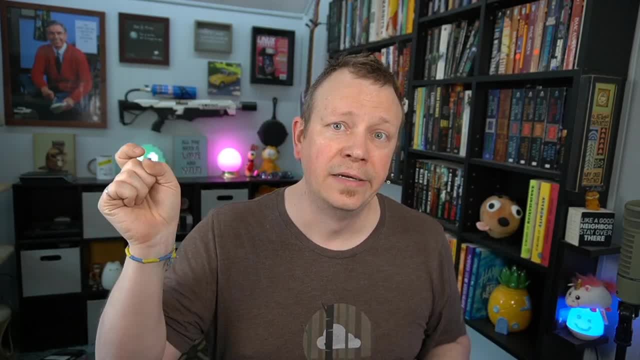 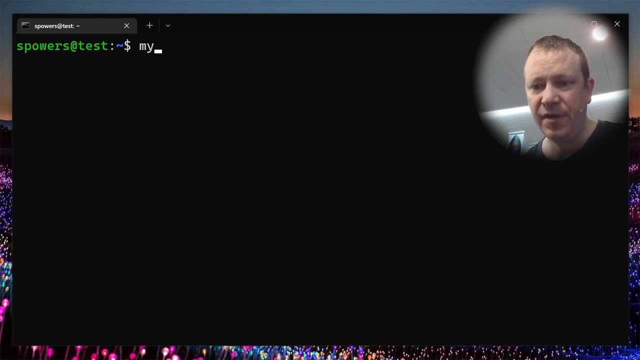 That's what you do, but I'm gonna show you how to do both on the command line right now. So the first thing I'll show you is our actual database system. Now I have Maria DB installed here, So I'm just going to do a MySQL dash U for admin, And okay, here's something that's. 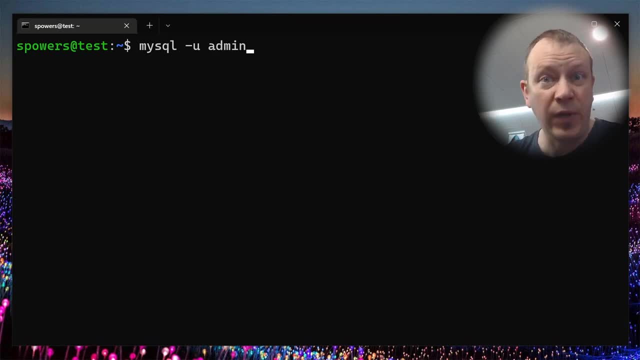 important to do when you are creating backups. with whatever method you use, you want to make want to have a separate user. Don't try to use the root account. It's good to have a user specifically for backups that has read access to all of your data And like if you're restoring. 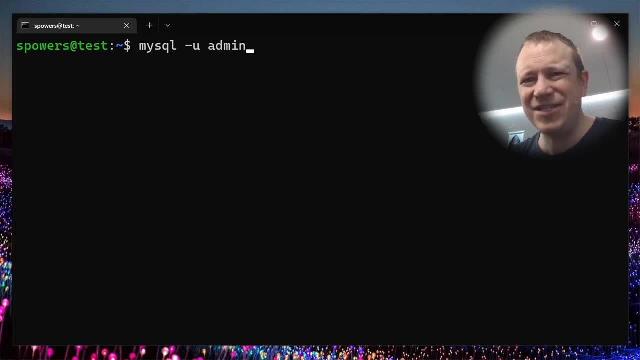 make sure it has right access and can create stuff. The reason is, using root is just not good practice anyway, And to have a specific user, a MySQL user, inside the MySQL server that you can access stuff makes things a lot simpler, because sometimes, especially with Ubuntu, 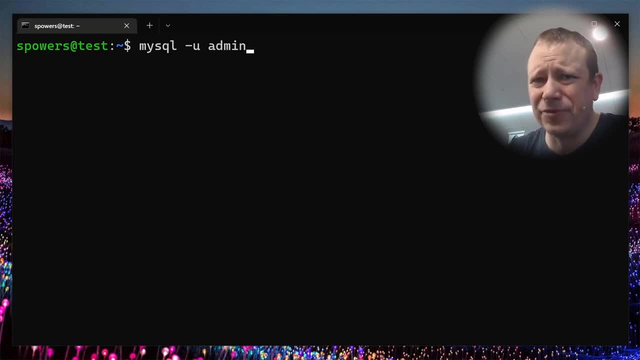 root user is weird. Like you don't use authentication for root. If you're the root user, it's weird. So not only is a good security practice, but sometimes it'll save you a lot of heartache. If you create a user in your MySQL or Maria DB database, that will give you access to it. 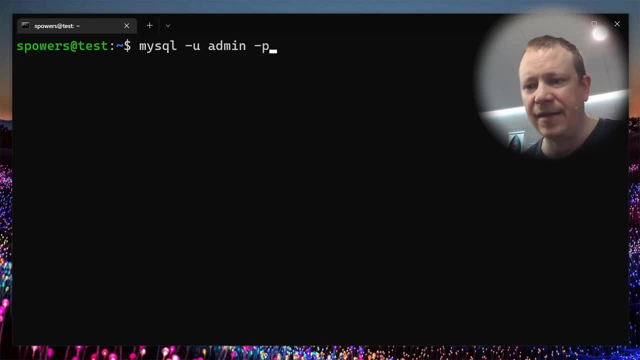 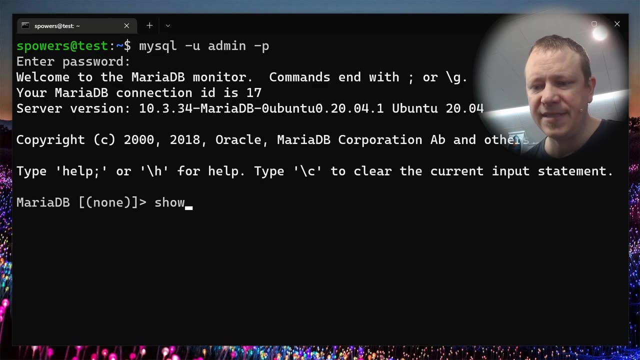 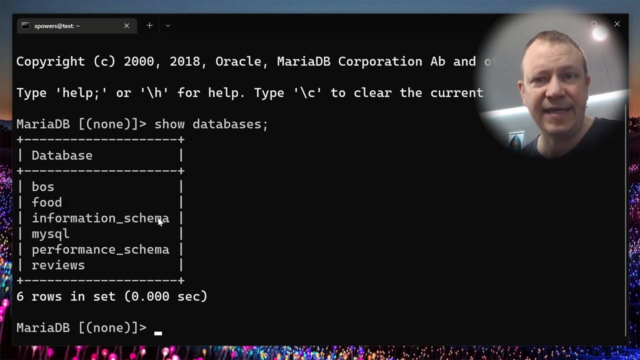 So my user is admin and my password is admin as well, which is not a great security practice, but this is just a test server. Now, what I want to show you is the databases. So show databases And you'll see. in here we have multiple databases inside the Maria DB and we're going to 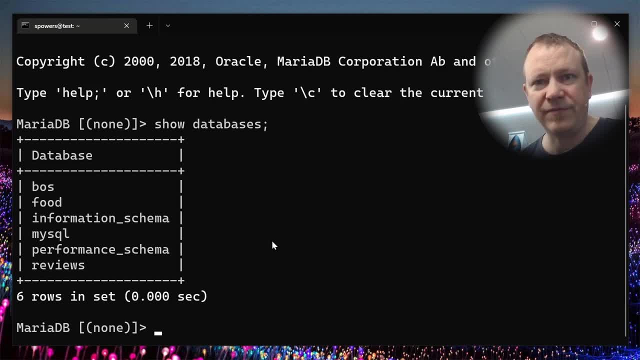 back them all up using two different methods, And I'll- even, if we have time, I'll- try to show you how to restore as well. So let's get out of here. The first thing we're going to do is use a tool. 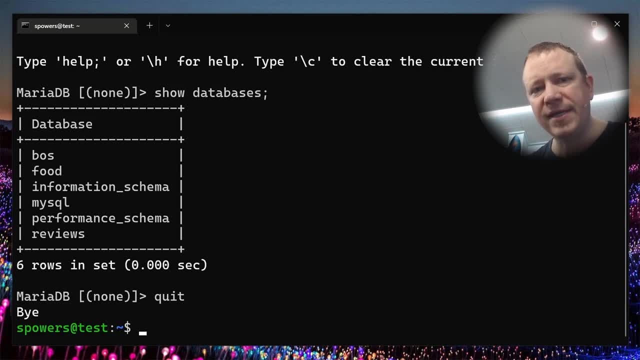 called Maria backup. Now I'm going to use pseudo because I want to uh make things simple. The the problem is, if you do it just as your user and uh the MySQL user has to have access to the folder, you can get some permission issues. So when you're doing this in production, 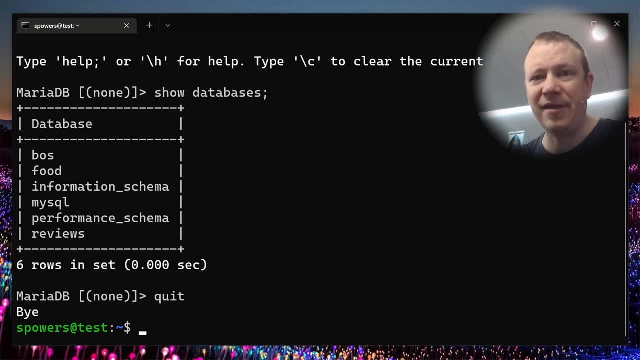 it's good to have a backup user who has access to you know the, the folders where you back up and stuff like that. I'm going to use pseudo for simplicity sake, uh, when I do this now. So pseudo Maria backup and I'm going to do dash, dash backup because I want to make a backup. 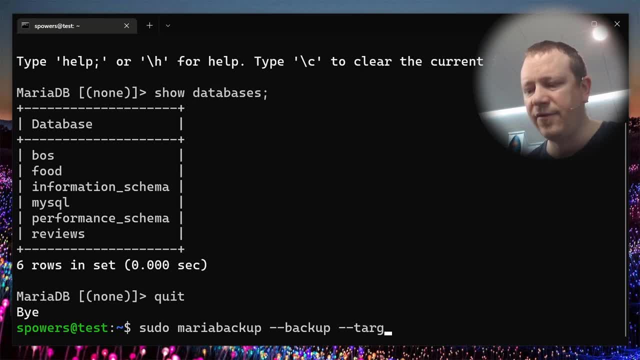 and we'll do target There we go. Target der equals and I'm just going to put it in my current directory: So home S powers and I'm going to put it in my current directory: So home S powers and I'm going to put it in my current directory: So home S powers and I'm going to. 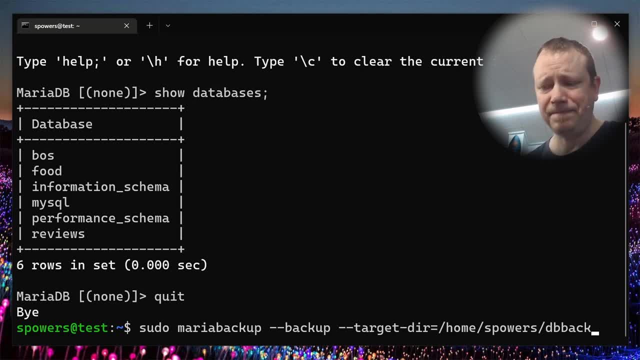 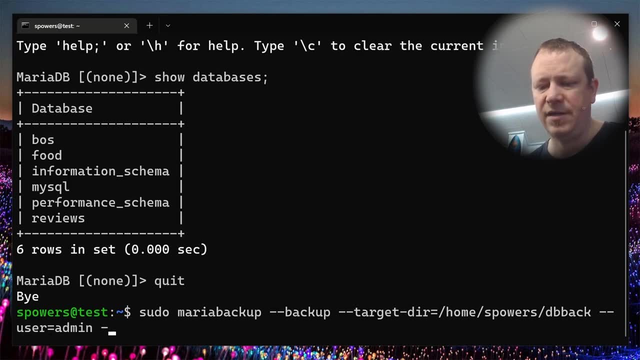 call it DB back. All right, That's the um folder that we'll create in my home folder. My home folder is currently empty. I have to say: user equals admin, dash, dash. password equals admin- again, poor security practice, but for what it is, that should work here just fine. And then we just press. 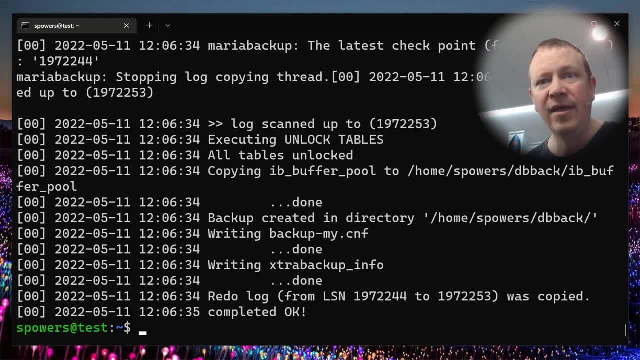 enter. Okay, It's going to go through and it's going to make a backup of all of my databases in a folder And remember, it's just making a physical, like file, copy of the var lib MySQL folder, But it does it in a way interacting with the server so that we don't get corrupt files. 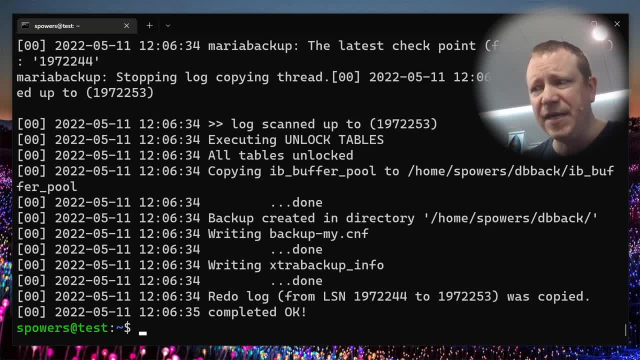 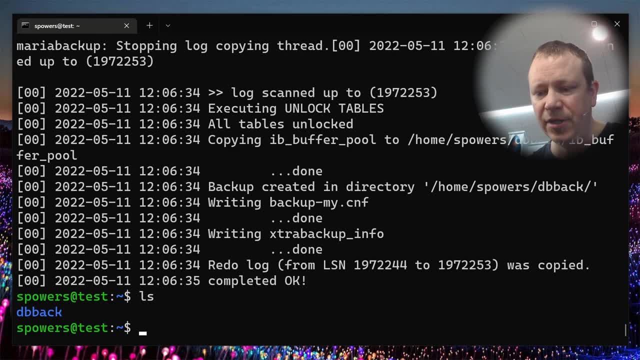 because, remember, we can't just back them up with regular backup software because they're actively being written to all the time. So this is a tool that goes in and just does magic behind the scenes to make it happen. So we look in here if we look inside. 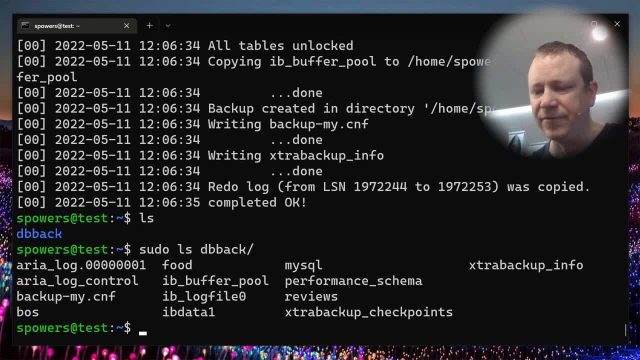 actually it's going to be owned by root. So sudo ls DB back, we'll see. just that's a copy of the MySQL folder. Now, what we also need to do is prepare this, and this is because of the way in ODB. 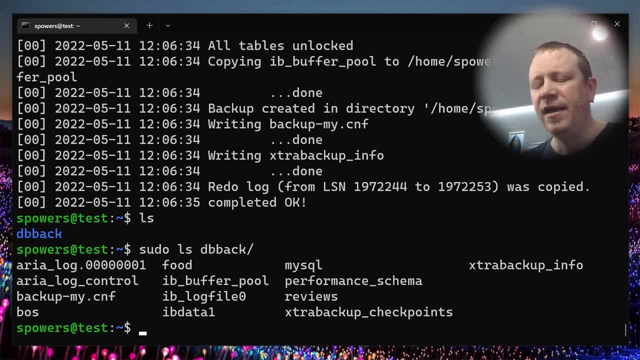 which is a format that MySQL Maria DB use. it does some weird things with timestamps and stuff. Basically, you want to prepare the folder that you backed up. I don't know why Maria backup doesn't do this in one step, But it's very similar. We just say: sudo Maria backup, This time instead. 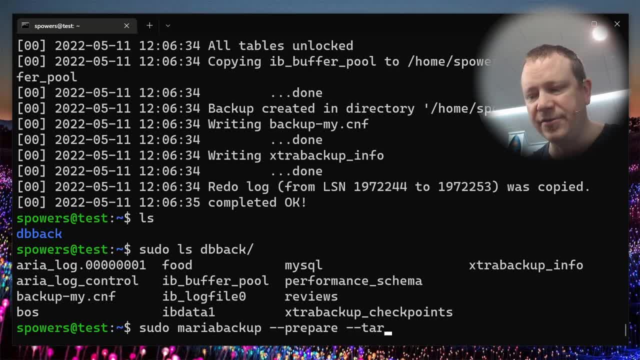 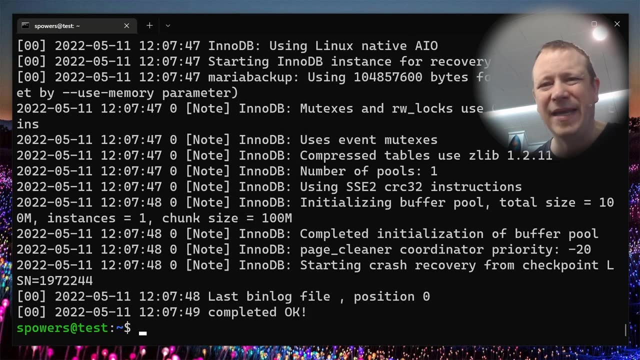 of backup. we say prepare And the target directory is home as powers db back And we don't need to authenticate to the MySQL server, So we don't have to put the user and password here. But we do this And basically what it does, it somehow makes configuration file. So the first time that your 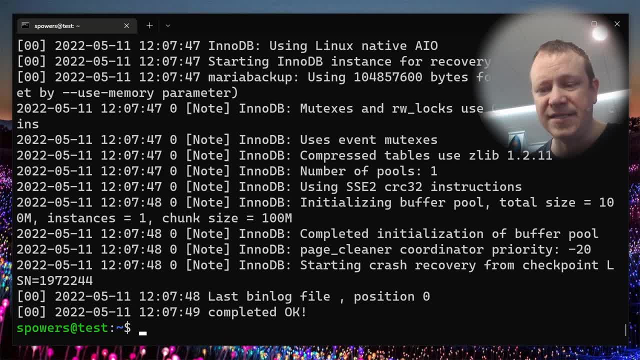 server sees this: if you restore it, it can. it can just automatically start working. Now You don't have to do this step until you're ready to import or restore, But because on a large database it can take a long time, it makes more sense to do the prepare step When you're backing up, when you 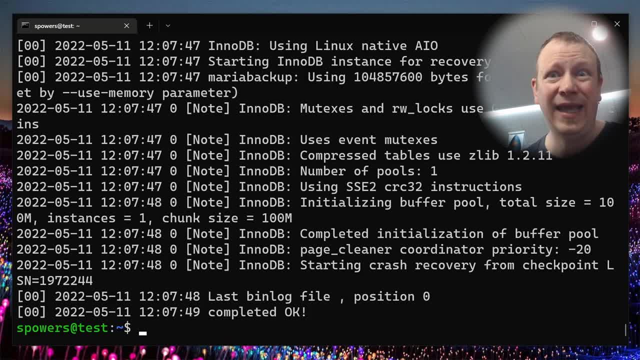 in the world, as opposed to- oh my gosh, the database is down and everything is falling apart. So rather than worrying about preparing your database, then I always do a backup and prepare in one step, so that it's ready to restore at a moment's notice. Okay, So anyway, we have the 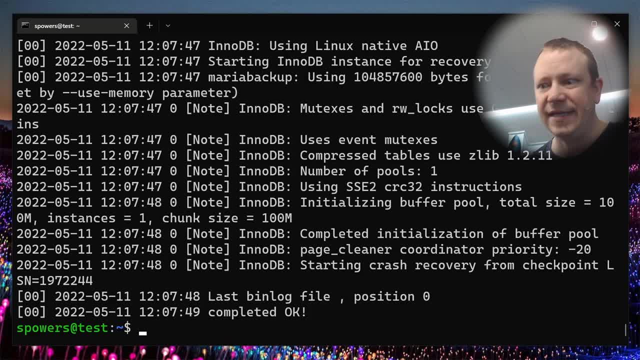 backup there and, um, to restore it. it's actually pretty simple. There's a couple of things you have to think about Now. we can make a backup without stopping the database. However, we cannot restore a backup with the database running, because we literally have to replace the stuff that is in. 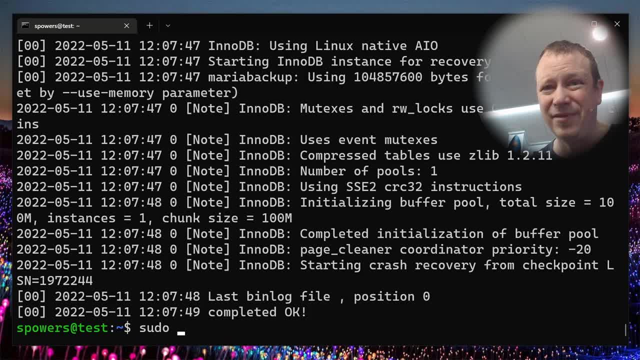 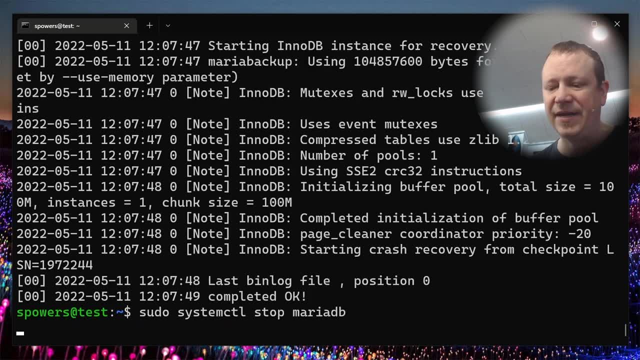 the in the folder. So the first step is to stop the database. So pseudo system CTL: stop Maria DB. It's going to stop the database. It's not running but theoretically everything is is hosed right now anyway. So it's okay that we're stopping it And then we have to go into 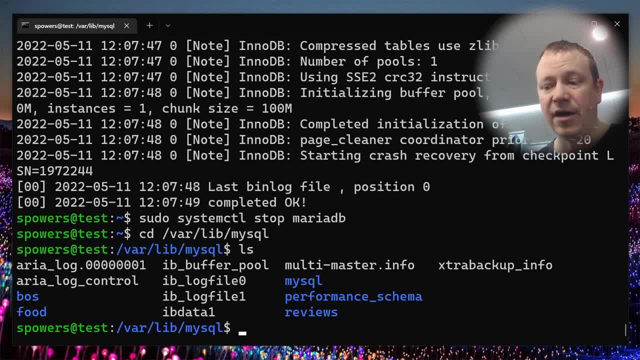 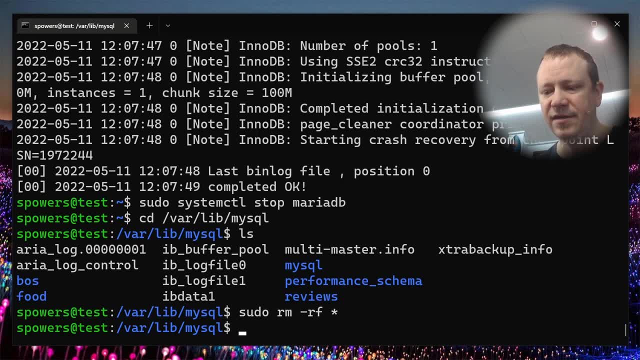 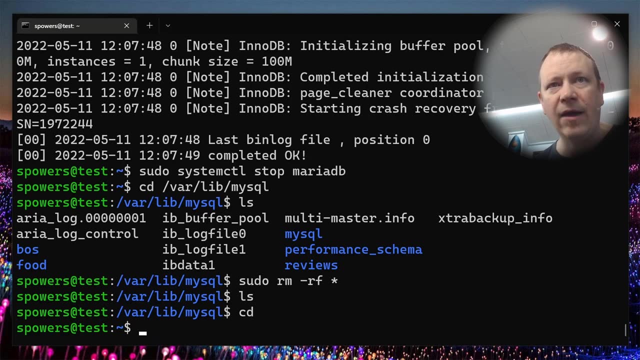 var, lib minus QL, And we'll see in here- these are the files that were- are supposedly now corrupt. So pseudo RM minus RF, star scary command, but nonetheless there's nothing in there now. Okay, So let's go back to our home director here and now we can restore it using 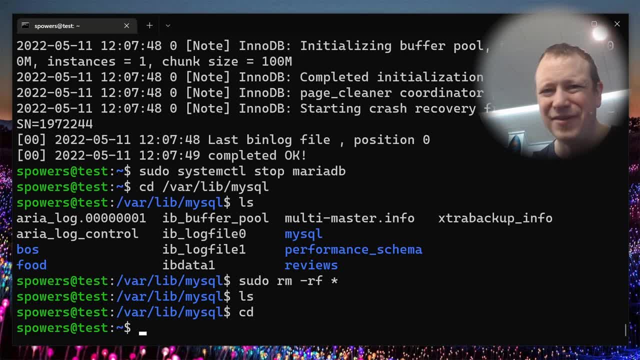 Maria DB. Now we can also just copy the stuff over. All this is going to do is copy it, but we can use Maria backup to do it as well. So pseudo Maria backup. dash dash, copy back. You can also do dash dash- move back. 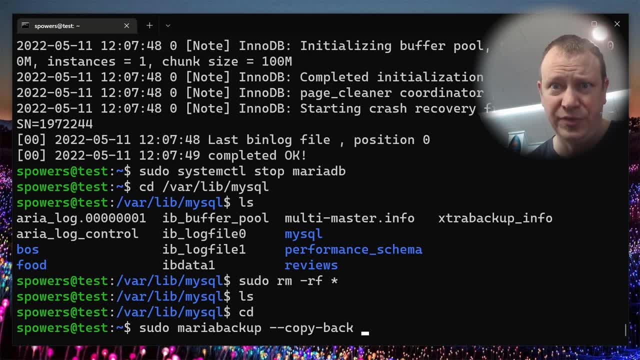 but I don't. I don't recommend that because it literally moves the folder and you've lost your only backup. So that's a weird feature to have. I guess, maybe if you're running out of disk space and they're huge. but anyway, I always do copy back to make sure I keep my original copy in case I screw up. 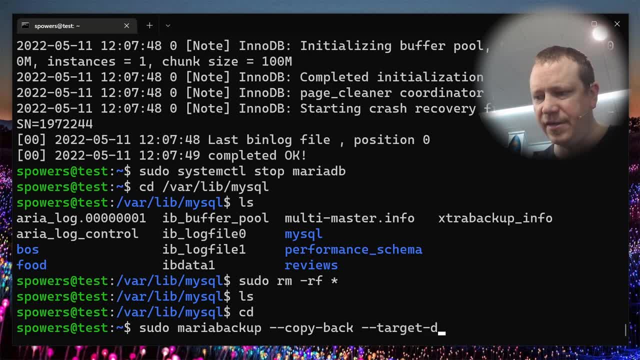 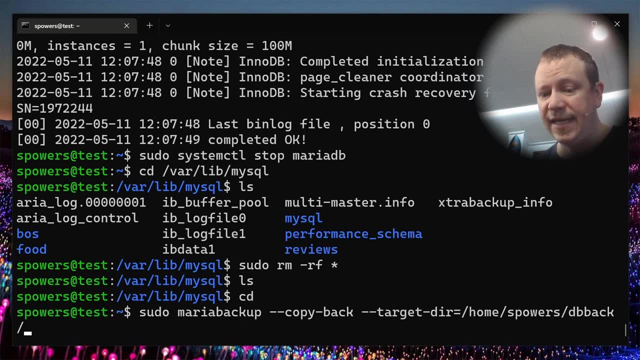 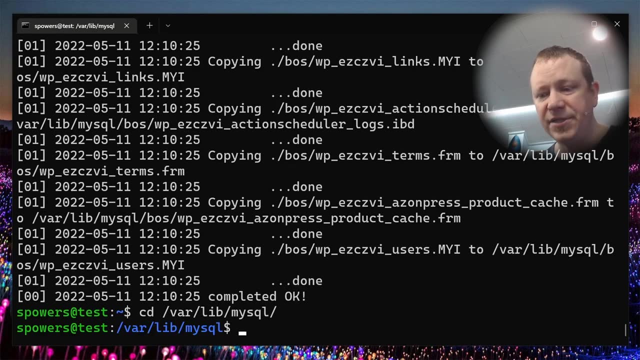 And then you say: what target directory? So target der equals home as powers DB back, And that should be all it takes. So we press enter and completed: Okay. And now, if we go into var, lib minus QL- the only thing we need to do now we look it's all owned by root, And that's no good, because it. 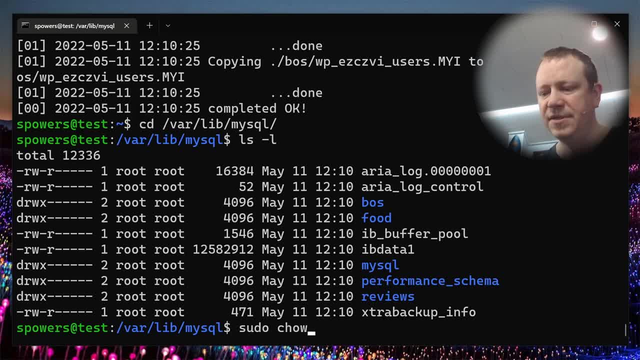 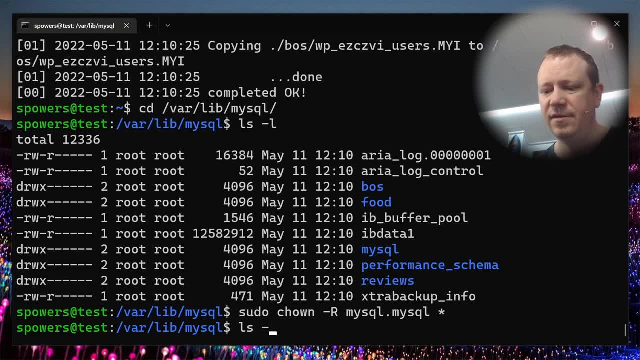 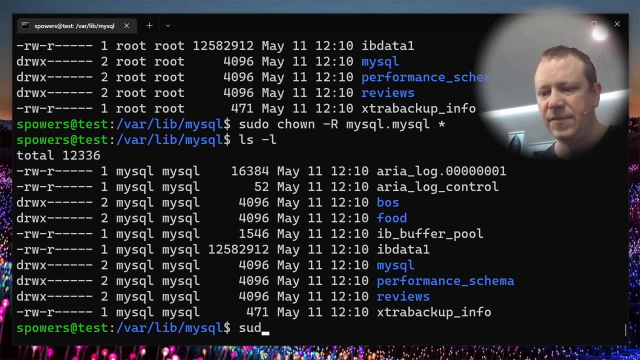 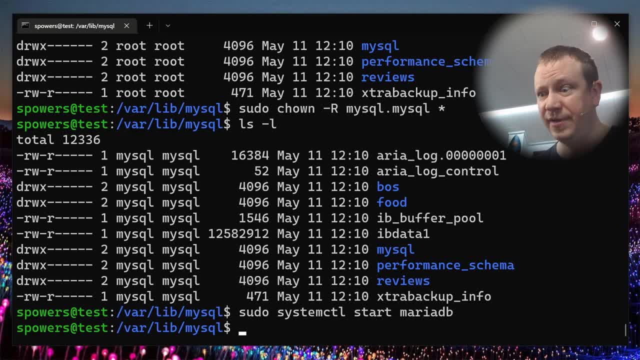 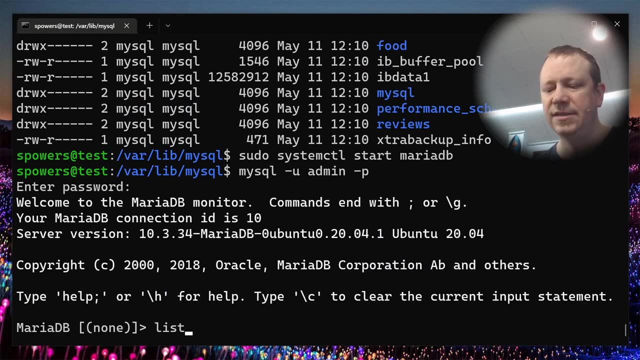 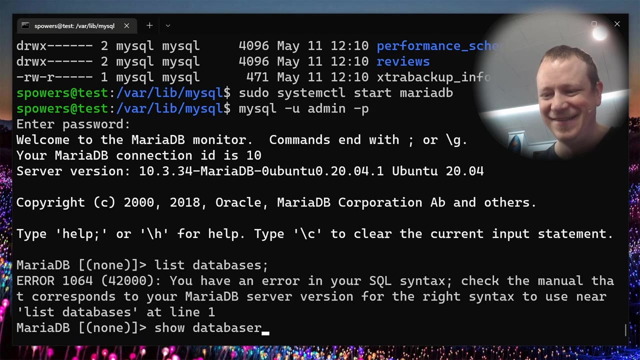 be all right. it started and now we should be able to have a fully restored and functional database. let's see: uh, mysql, dash user, admin, dash p. prompt me. admin and moment of truth database: sorry list databases. it's not listed. show, show databases. and there, now we have all of our databases back. everything was restored from that backup and 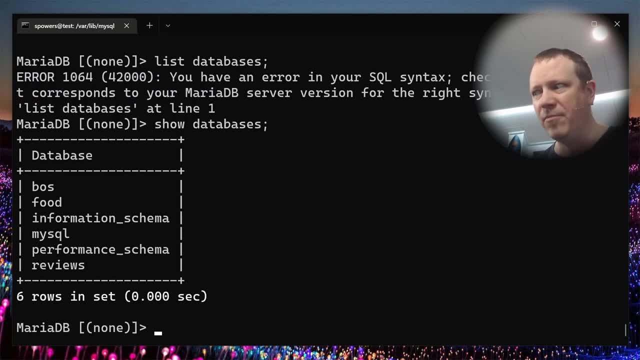 that's how you do a physical backup and restore again. in the moment it's probably going to be a little bit more panicky because everything is down etc. but if you have a good backup, that's how you restore it. you just have to remember those couple things. it has to be prepared. 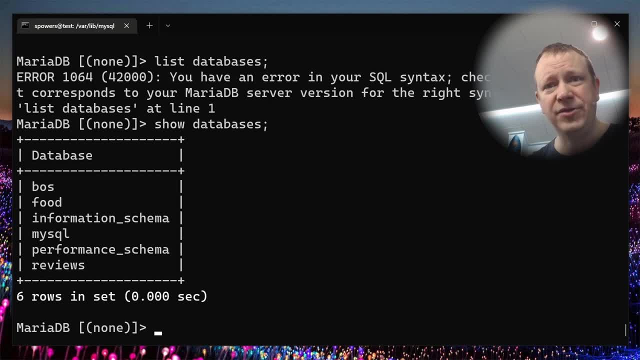 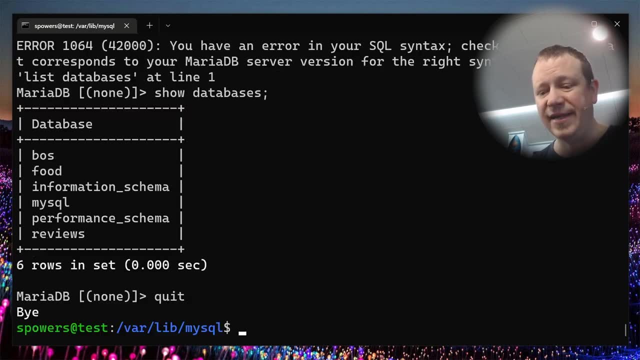 uh, you have to make sure to ch own it back to the database users ownership to make sure that it owns it and it can, you know, read and write to the files and that's really all there is is And that is a physical backup. Now, really quickly, we do have time here, So I'm going to 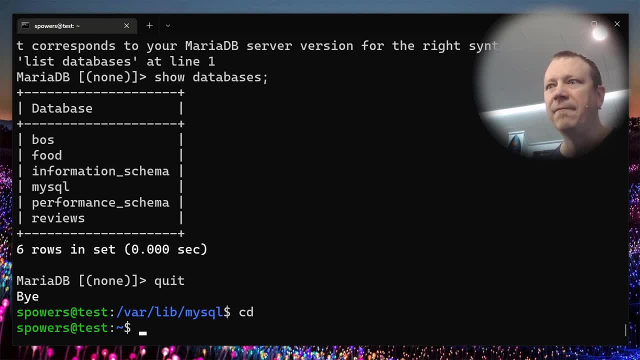 show you how to do a logical backup as well, Because it's not really difficult And for some cases it's really really useful. So in this case, I'm going to say: sudo minus ql, dump dash u for user admin, dash p, admin- again my admin, admin account, And I'm going to say all dash. 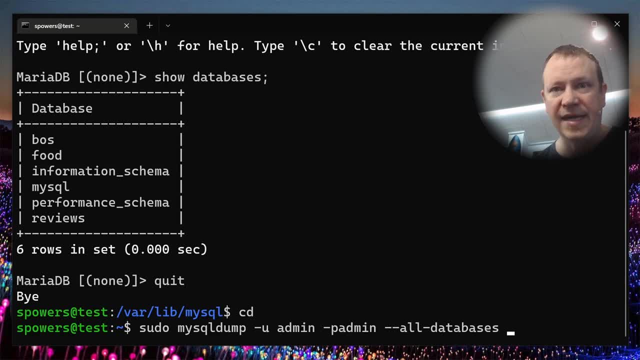 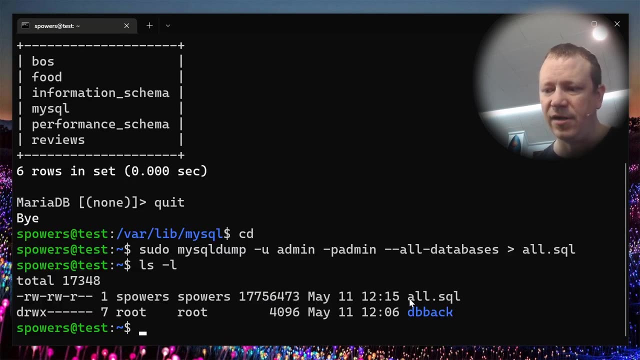 databases And that will create a MySQL dump of all the databases, but I want to redirect it into allsql. Now we could redirect this to gzip as well and have it compress on the fly, But we'll just do this And now, if we do ls minus l, we'll see we have now allsql And this is our entire. 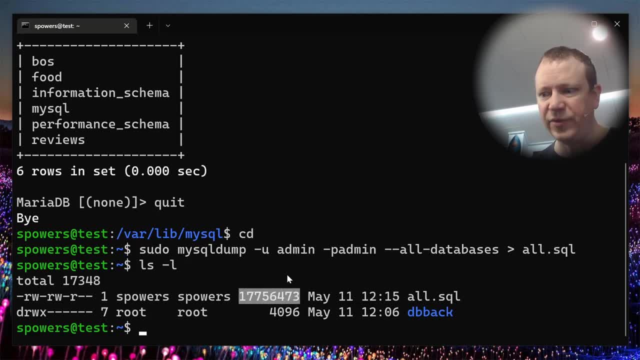 set of databases that are in our MariaDB as one single SQL file. So we could re import that in if we wanted to And get all of our databases restored, But it's really nice to just do one database. So let's say that my BOS database got corrupt And that's my brain of Sean blog that I actually imported in. 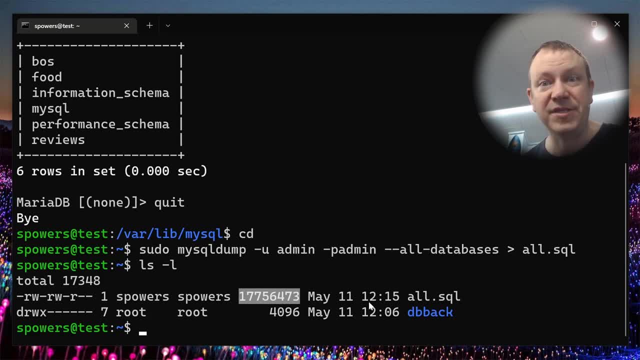 this test, just so we'd have some stuff to work with. Let's say, that got corrupted, So I could say, Okay, I know I have a good backup, So let's delete the bad one And we don't have to stop. 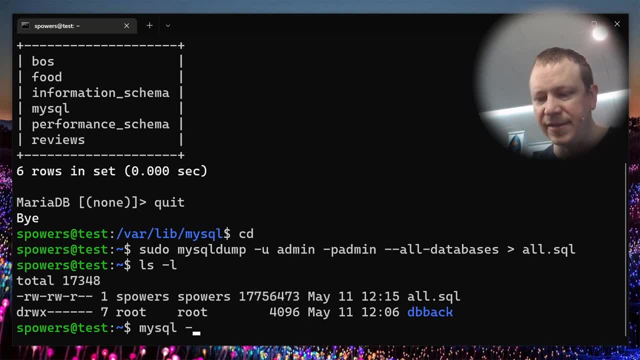 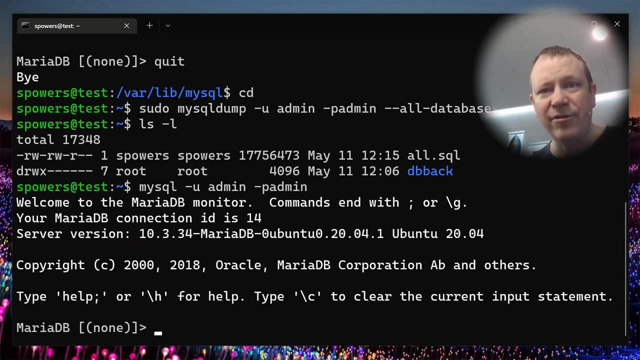 MariaDB. In order to do this, all we have to do is say MySQL dash u admin, dash p admin. So we're in here now And I can say: All right, know that right now the brain of Sean database is bad, So I can just say drop. 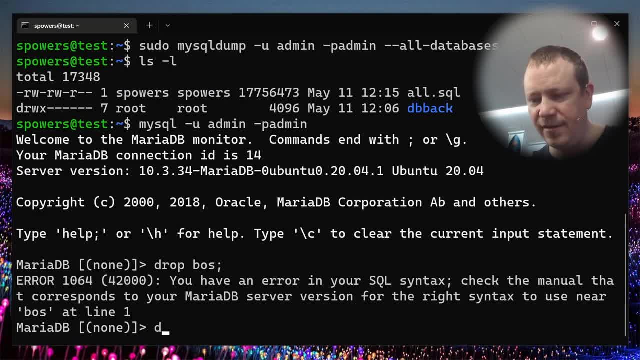 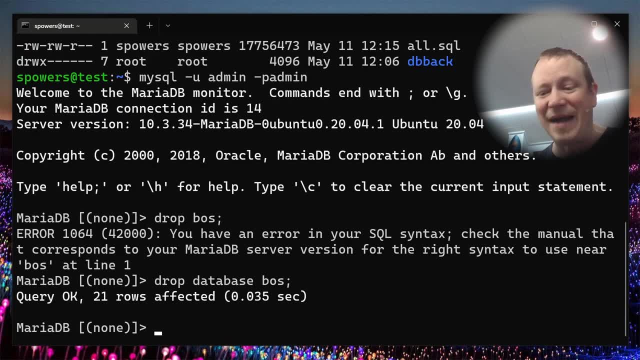 us- And I am not good at this syntax here- drop database BOS there. Okay, so we dropped the database completely. there is no more BOS database in our MariaDB. we need to create a database, just an empty one. So there's somewhere to import our backup to. So I'm just going to say: 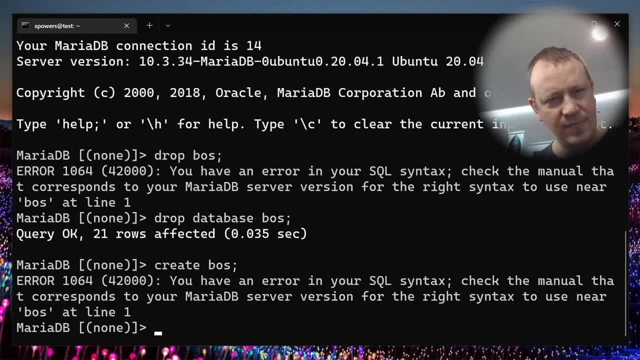 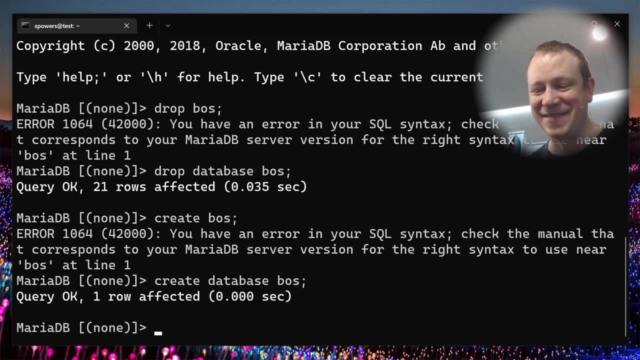 create BOS Again- boy, I'm bad at this. create database BOS. Okay, so we've created a database. it's empty, there's nothing in it. But let's quit and change that. Now, all we need to do in order to populate? 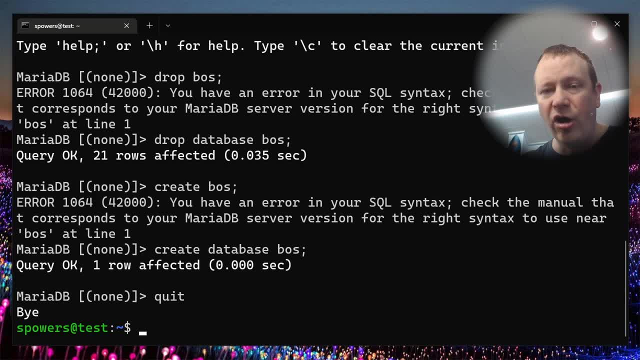 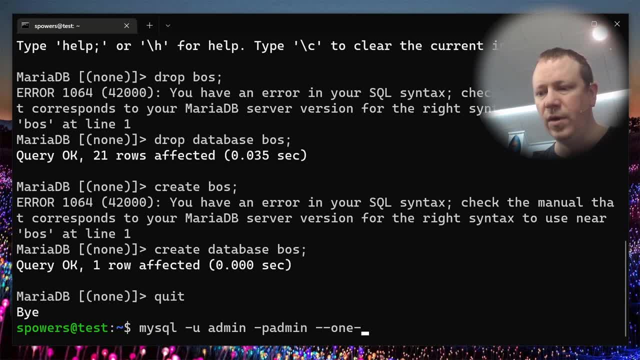 MySQL: dash u admin. dash p admin. MySQL dash u admin. dash p admin. MySQL dash u admin. dash p admin. one database which is telling it. we just want to do one database, not all of them, And the one database is BOS, So we want to import this one database. 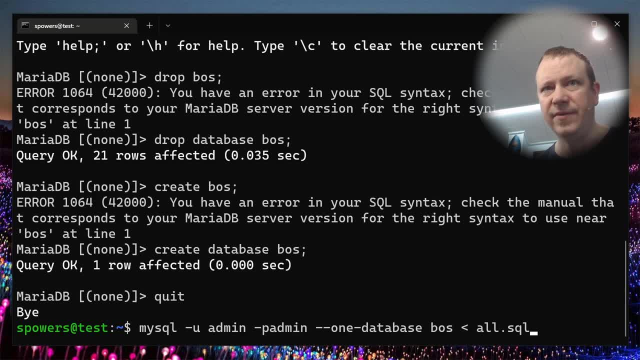 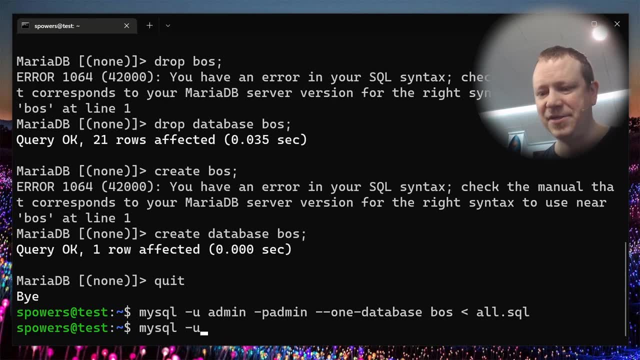 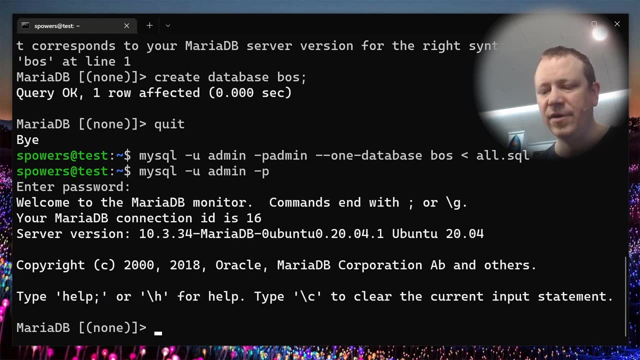 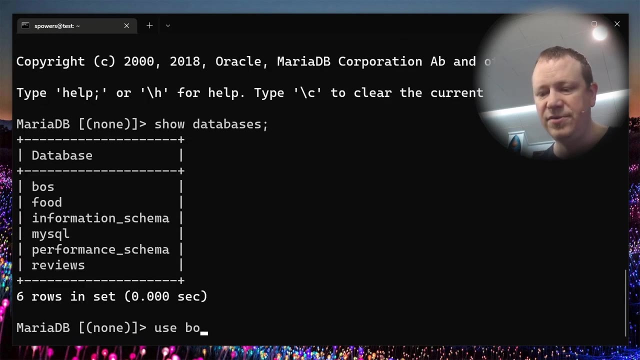 and less than we import it from all that SQL Notice, the server still running, press enter And now MySQL dash u, admin dash p. Now if we do, I'm going to say well, if we do show databases, we're going to see that of course BOS is there. I'm going to say use. 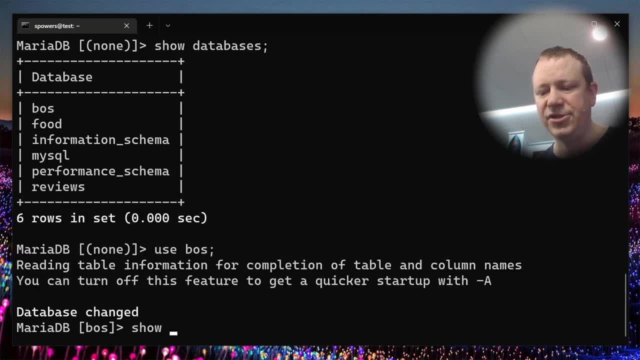 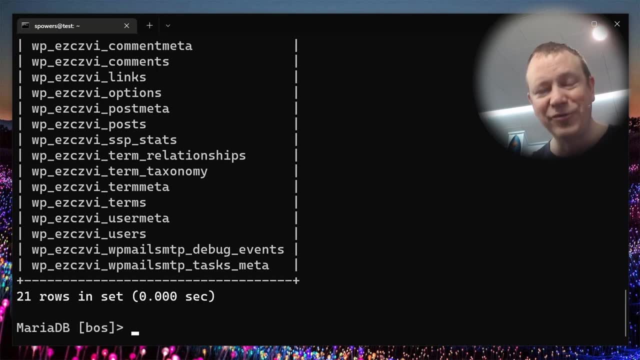 BOS. Alright. so now I'm in there And I can say: show tables And look, our database has been restored. Remember we dropped it and created it empty, But now it's been recreated and restored from that backup. It's actually super, super cool. Now, while we're on the command line here, 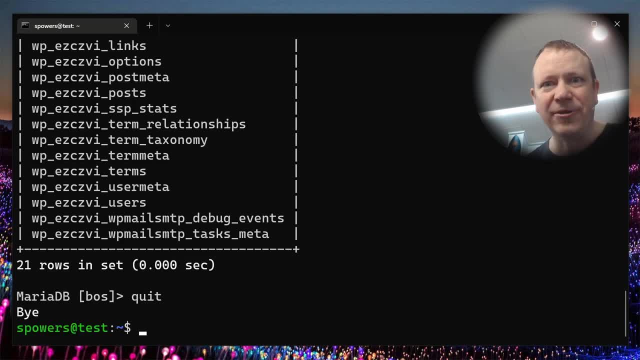 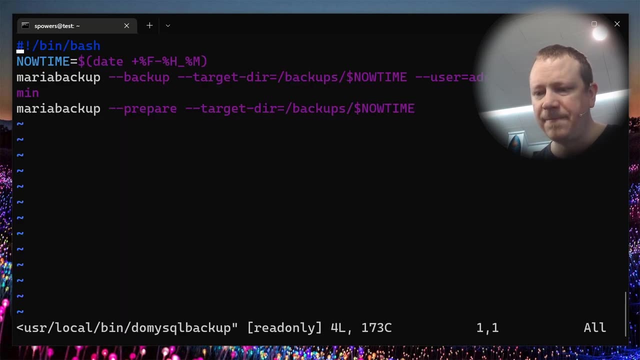 let me get out of MariaDB. I do want to show you when I do a physical backup with MariaDB, I I'm I tend to automate it, And so just a simple automation script might look something like this: So, user local- I had just one that I I scrapped together been. So something like this I would say: 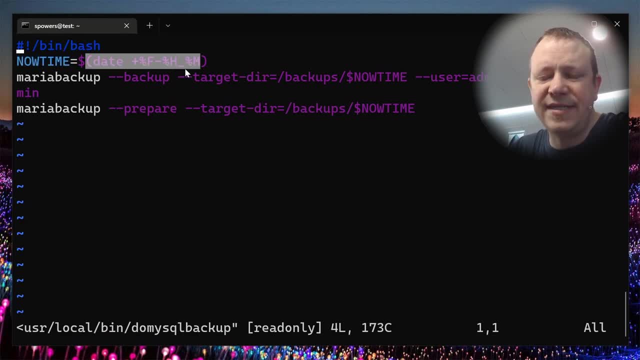 set a variable, now time to the date, And this is just a date that has the month, day, year and then dash hour in the minute, And it does a backup with a target directory of that date. So like backups, so I can do. 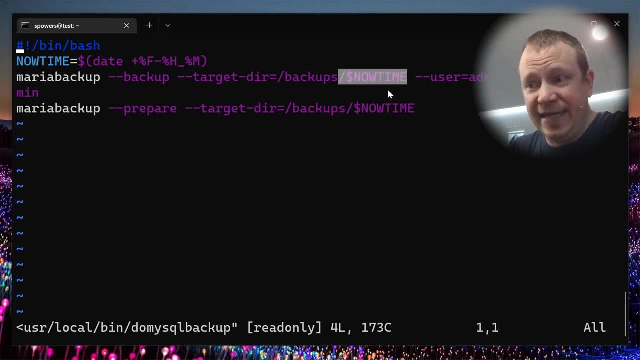 multiple backups, because it's just going to make one based on the current time user admin, and then the next step is going to be prepare that target directory that we just did. So it's ready to restore as well, And I just do this regularly And then I'll have regular. 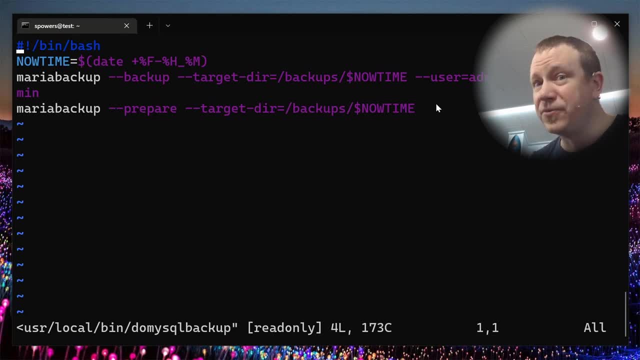 backups automated using cron So that if something goes wrong, I can go back to either the most recent or the most recent before things went sideways and have those to restore, And you can do the same thing with a logical backup. you can start a backup with a logical backup, you can. 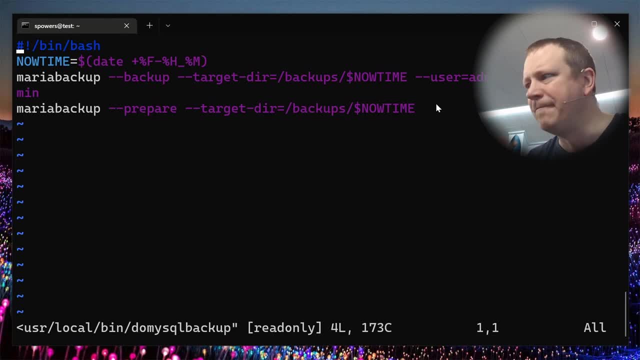 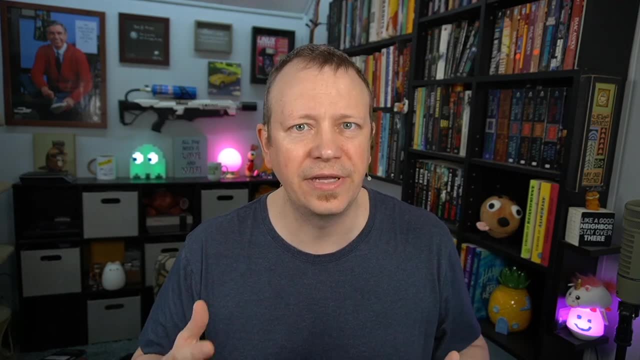 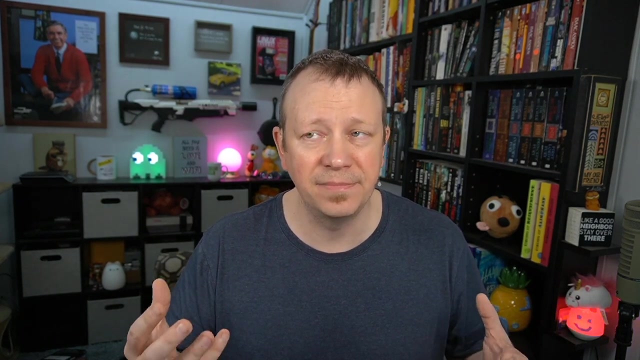 script it and have it create those backups on the fly, compress them, rotate them, all of those things. So again, we know backing up everything is very, very important. But it can be a little more complicated with databases because they're always in use And you can't back them up with. 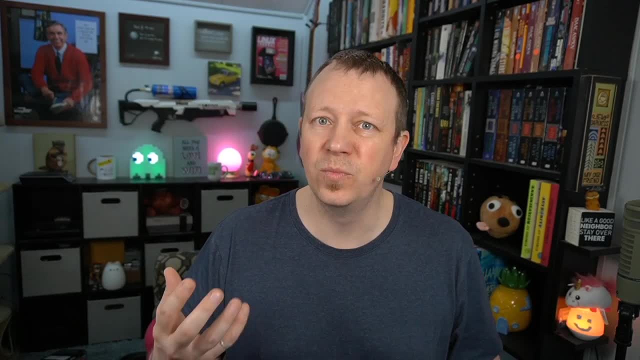 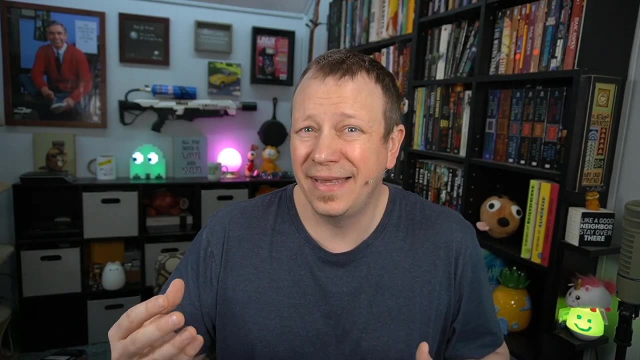 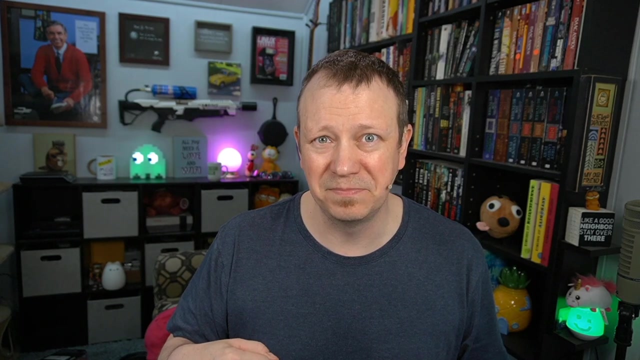 traditional backup tools generally. So having some ways to do that and automate it is really, really important. Hopefully this video cleared up the different ways you can back them up And you one of these backup processes into your own cron system, backup system And gosh. I hope you have.